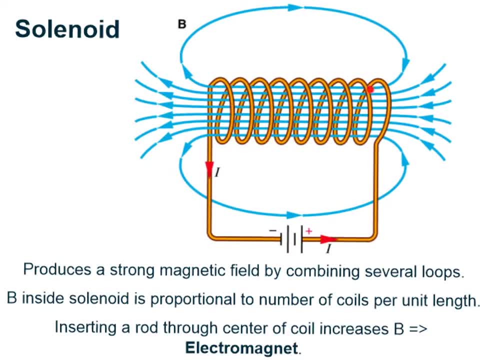 and you can see the direction of the magnetic field. You can see the picture of that here. Here is our solenoid. multiple loops and a very strong magnetic field can be generated this way. Inside of this solenoid the magnetic field is extremely strong. You can see those magnetic. 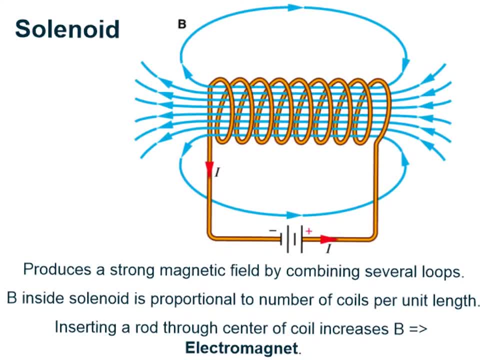 field lines are very close together, indicating a very strong magnetic field. The strength of the magnetic field inside of the solenoid is going to be proportional to the number of coils per length of wire. And also we can do something else. We can insert a rod, We could put a metal piece, a nail. 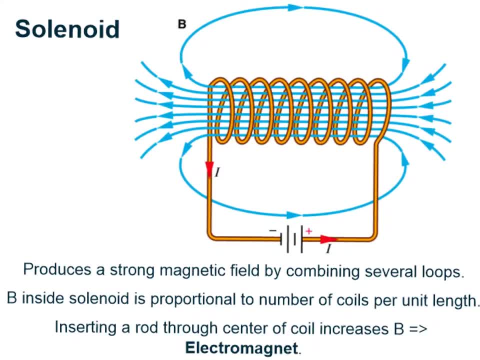 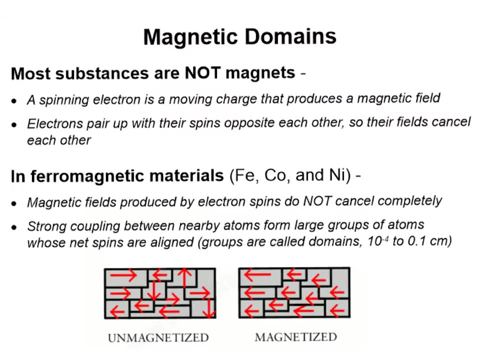 if you have a nail through the center of the solenoid, and we can increase the magnetic field strength even more, Doing that is what we call an electromagnetic magnet: inserting a piece of metal inside of that solenoid. Now let's talk a little bit about 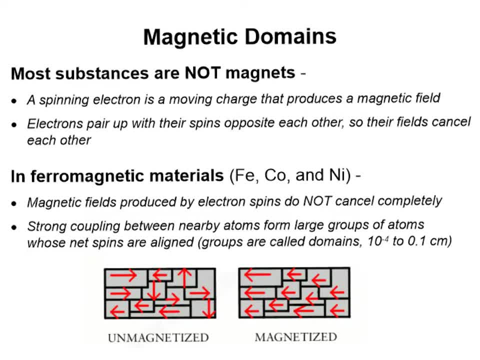 what we call magnetic domains. Most substances you'll notice, are not magnets. Most substances cannot be magnetized and the reason is, if we start to think about things on an atomic level and think about the electrons involved, if we have a spinning electron, 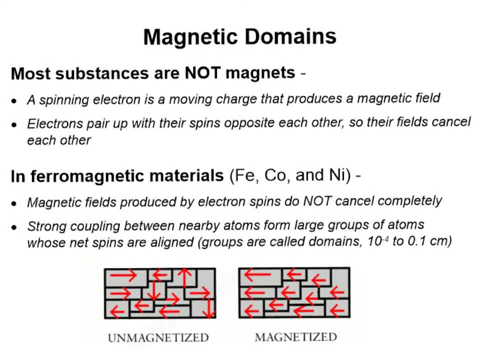 that spinning electron is a moving charge and it is producing a magnetic field. that little electron. When we talk about most substances, most substances have electrons in their atoms that are pairing up with their spins opposite each other and so their fields cancel each other out. So most 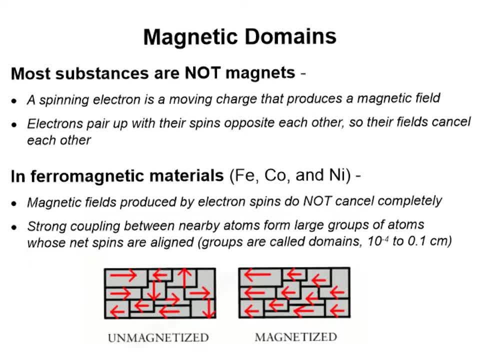 substances are not magnets. There are some substances that we call ferromagnetic materials- iron, cobalt and nickel would be some of those- And in these materials the magnetic fields produced by those electrons spin together. they are magnetic. So if we start to think about this, 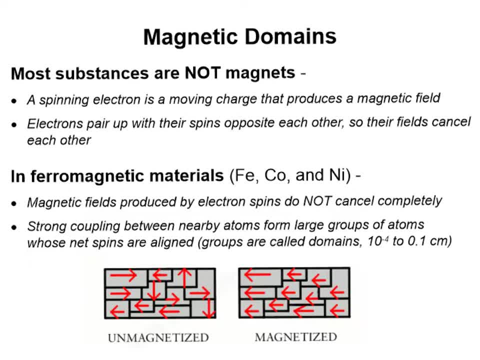 Spins are not completely canceling each other out. In fact, there's a strong coupling between nearby atoms and it forms large groups of atoms whose net spins are aligned. We call these groups of atoms domains. They can be anywhere from 10 to the negative 4 to 0.1 centimeters in size.